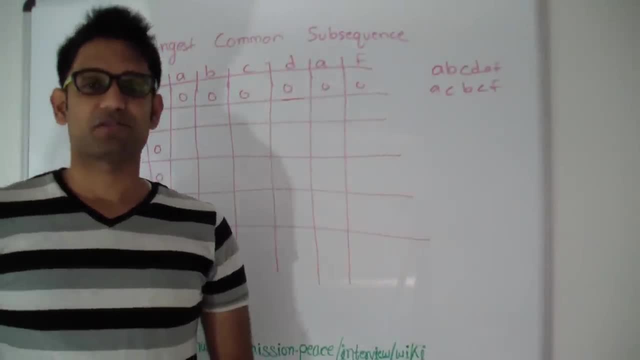 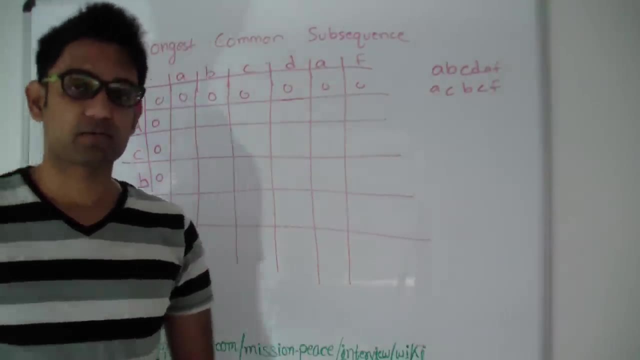 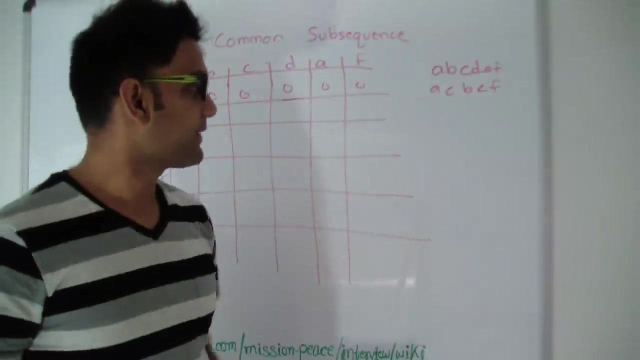 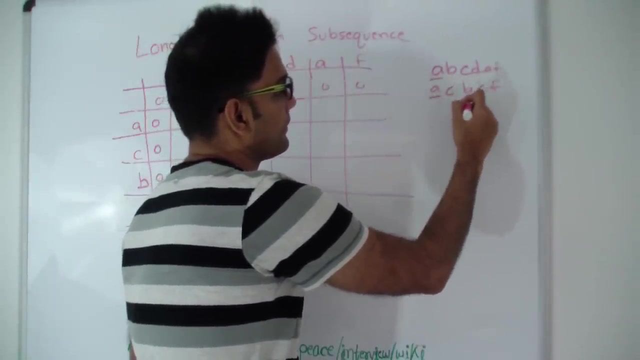 Hello friends, my name is Tushar and today we're going to look at the question longest common subsequence. What is this question? Given two strings, how do we find the longest common subsequence between them? So for this particular two strings- A, B, C, D, A and F, A, C, B, C and F- the longest common subsequence will be A, A, B. 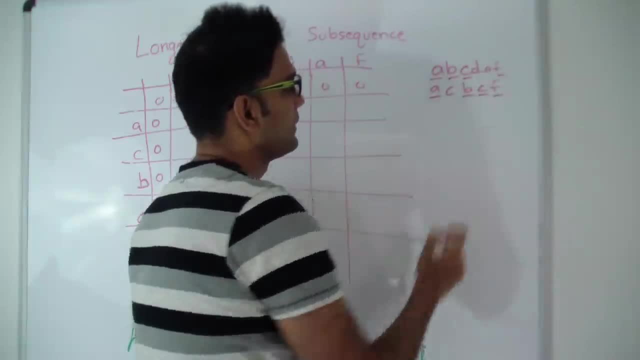 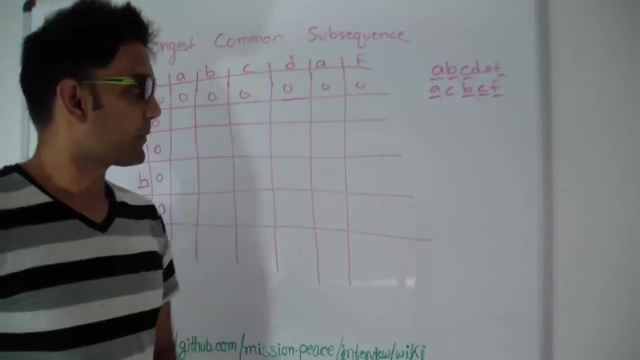 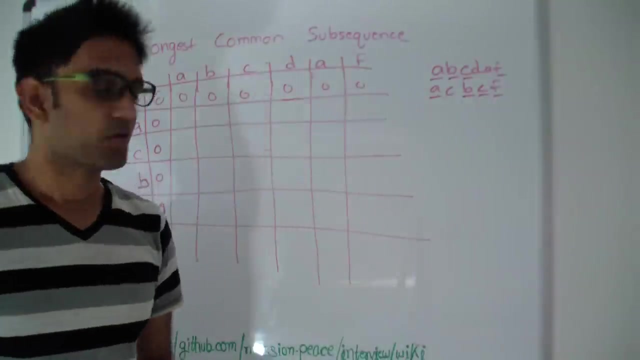 B, C, C, F and F. So the length of the longest common subsequence will be 4 and the longest common subsequence will be A, B, C and F. So the thing with subsequence is that it need not be continuous in the string. So here A, B, C and F, and we ignored C. 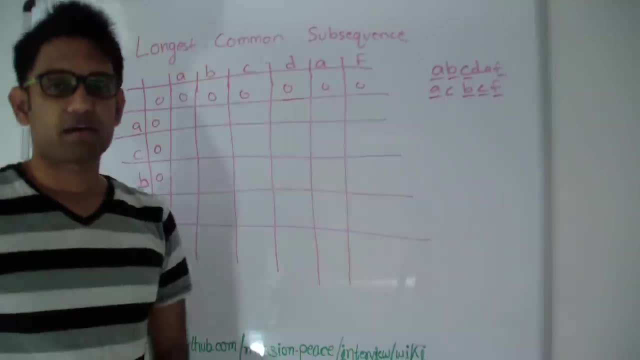 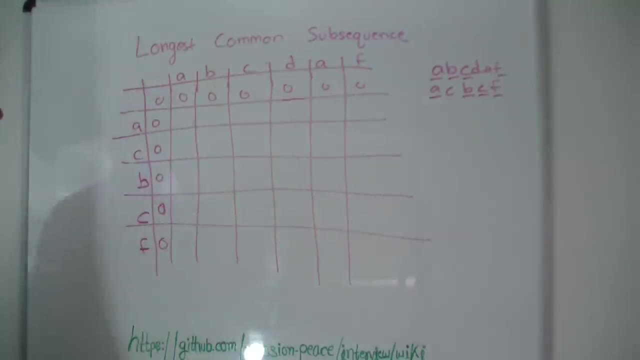 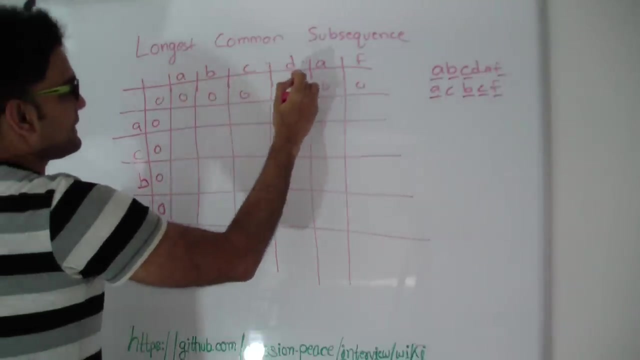 and above A, B, C and F, and we ignored couple of characters in between. So how do we find the longest common subsequence? Yes, we will use dynamic programming to solve this question. So here I have. on the first row I have the first string: A, B, C, D and A and F. On the first, 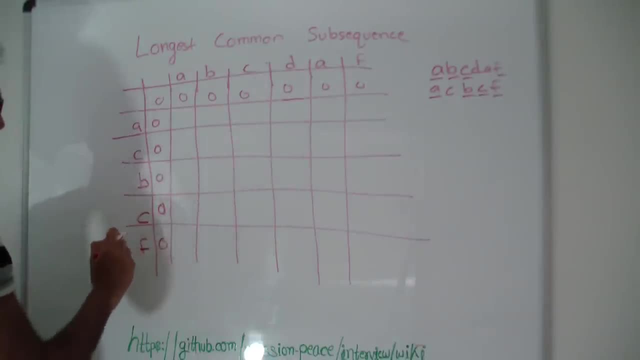 column I have the other string, A, C, B, C and F, Second row and second column are just populated with zeros. Alright, so now let's fill this matrix and finally, we'll have our solution when the matrix is totally filled. So when I'm filling this particular point in the 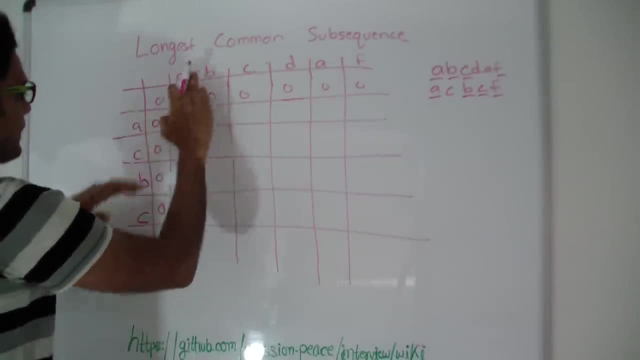 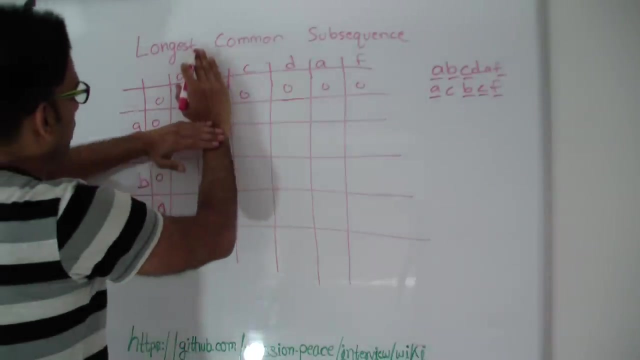 matrix. I'm asking myself if I had a string A, B, C and A and nothing else, What will be the longest common subsequence here? So the length of the longest common subsequence here will be 1, when I have just these 2 guys. 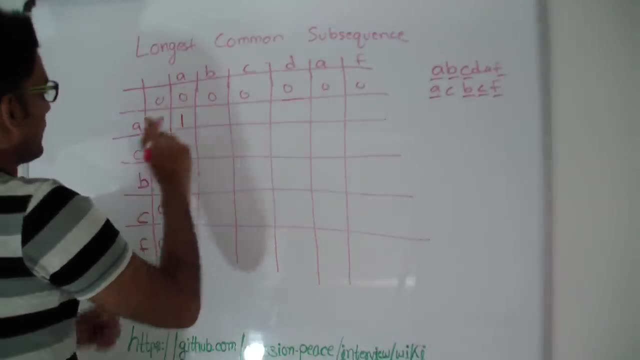 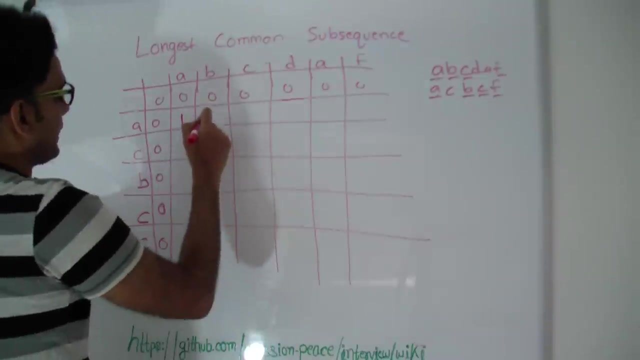 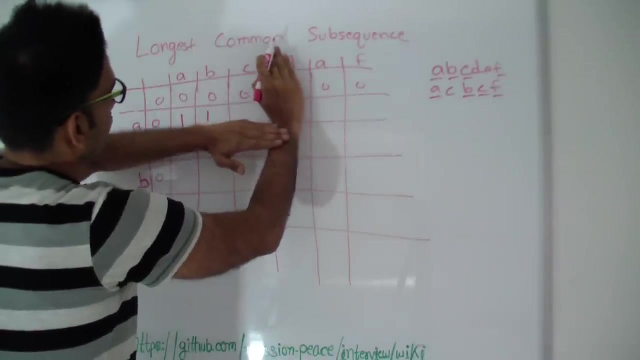 So 1. Now I have string A and B and A. So if I string A, B and A, what is the length of the longest common subsequence? here Again, of length 1. When I have string A, B, C and A, what is the length of longest common subsequence? here Again, length 1.. 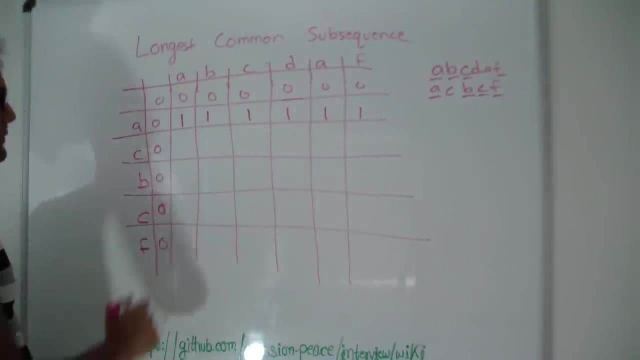 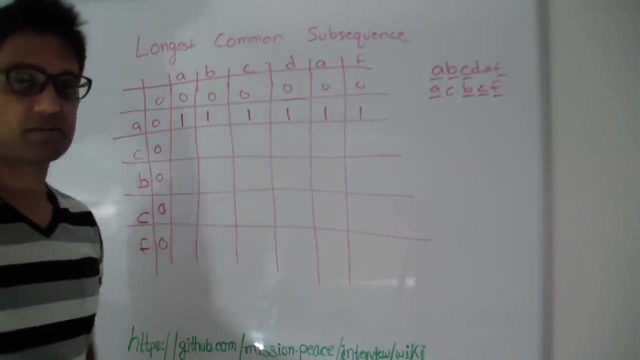 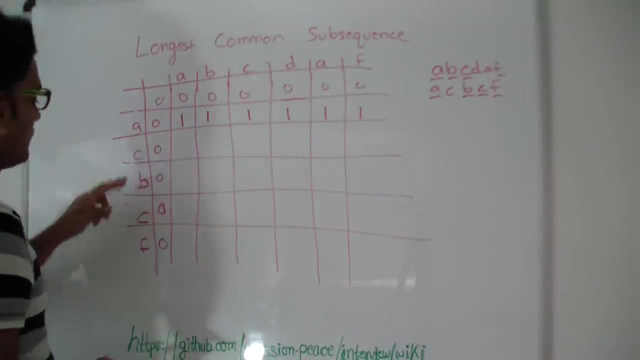 1.. 1 and 1.. So if we had string abcda and f on one side and just a on the other side, the longest common subsequence, there will be a. Now we'll fill for this second, second, second, third row, which is, which is, which will now include c. So here, 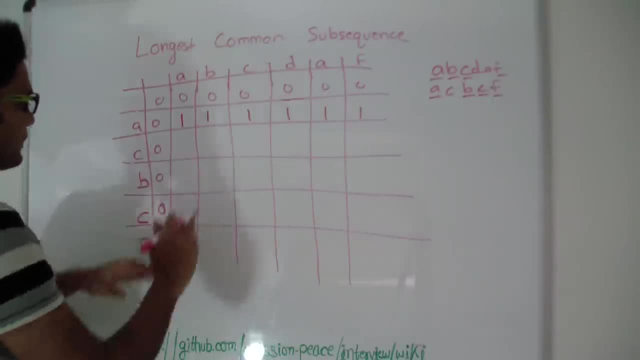 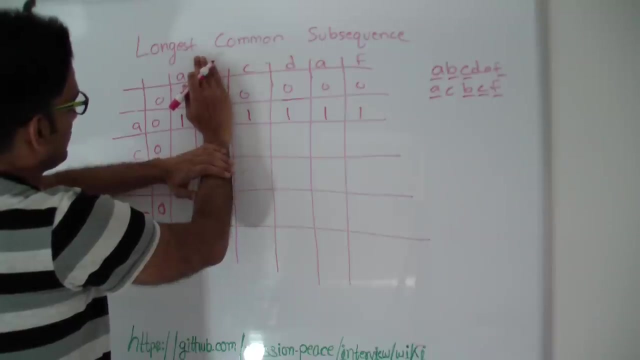 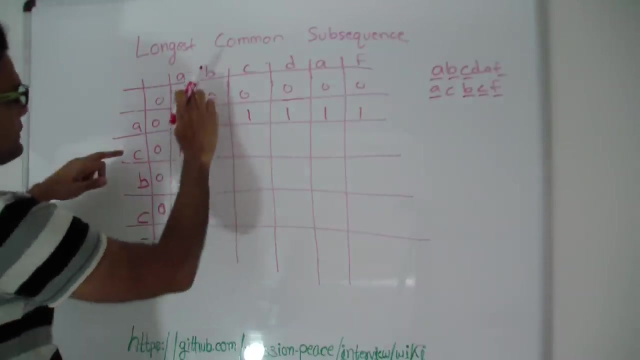 we'll have a and c on one side and a on other side. So you'll ask yourself, if I had string a and c and a, what is the longest common subsequence? here Again, 1. Where did we get this 1 from? From the top. So what we are seeing is, if these two 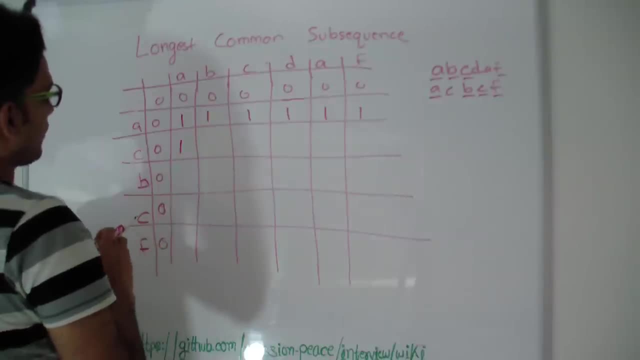 guys are not same, then the length of the longest common subsequence will be either max of the guy at the top or the guy at the left. In this case this is 1, so it it becomes 1.. We have string ab and ac. What is the length of longest common? 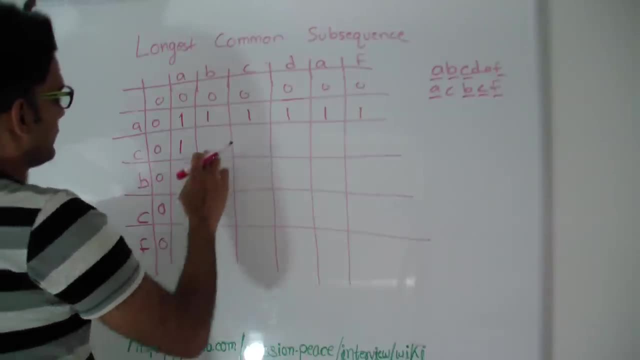 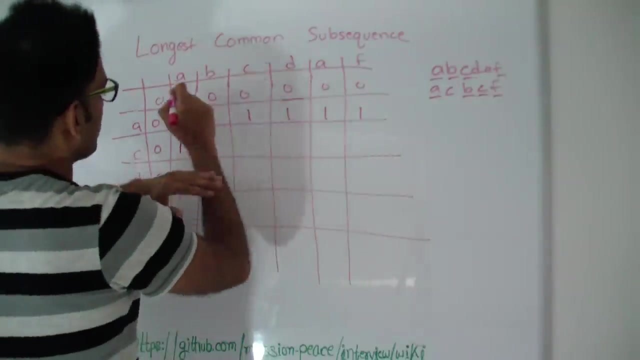 subsequence here. Since c and b are not same, the value here will be either the max of this or this. So in this case it's again 1.. Here we have string ab and c and a and c. Now c and c. 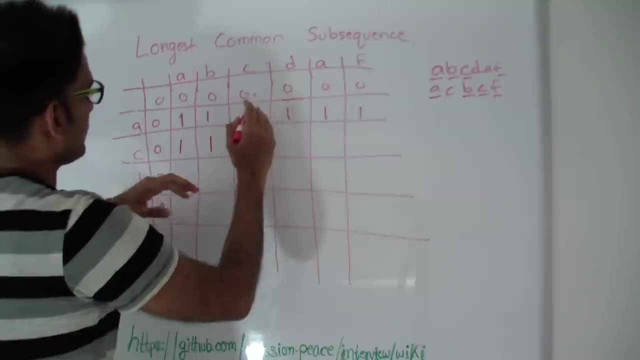 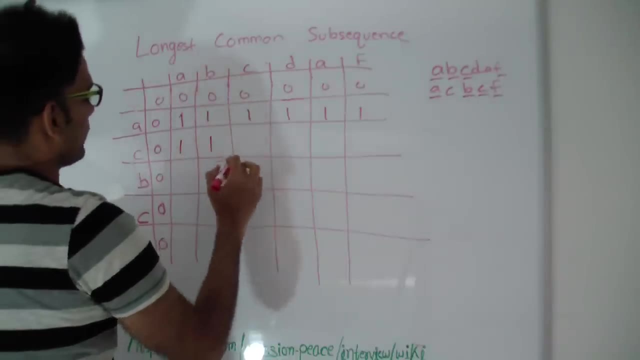 are same. So the length of longest common subsequence will be 1, because c and c are same, plus whatever the best we did between ab and a. So this one, So 1 plus 1,2.. So again, if these two guys are same, so the length of the longest common. 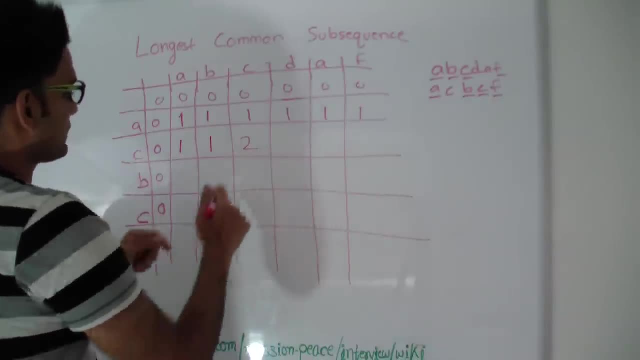 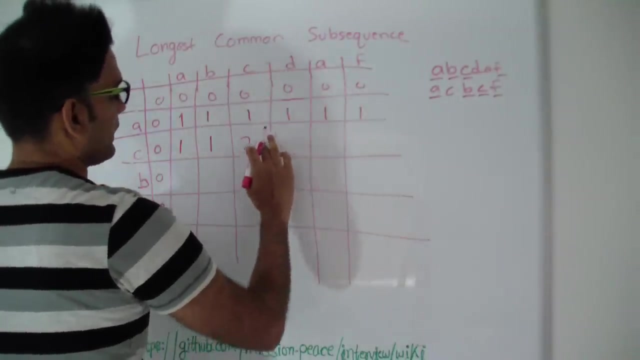 subsequence will be this plus 1, and if they're not same, then the max of this or this. Let's fill d in the same way. So since c and d are not same, we get the value from here, so 2.. 2 and 2.. 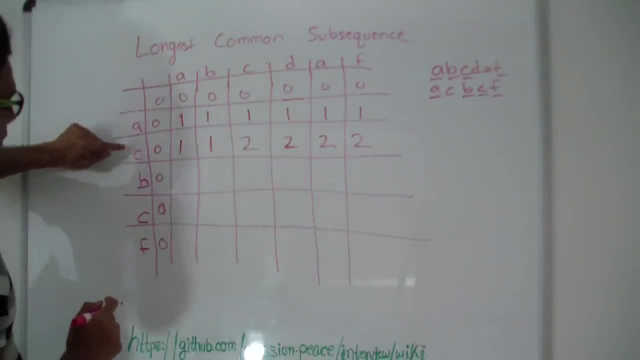 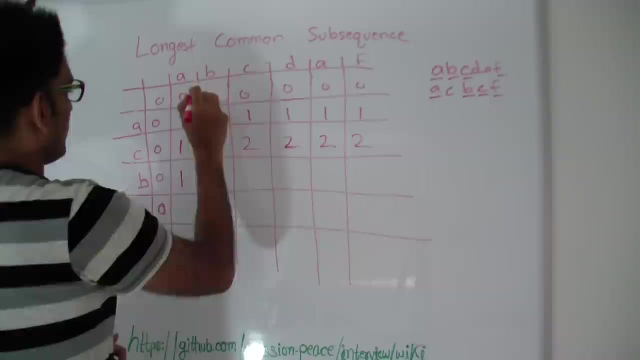 Alright, let's move here. If you had string abac and b and a, the length of the longest common subsequence will be 1, the guy from here. For now b and b are same, So the length of the longest common. 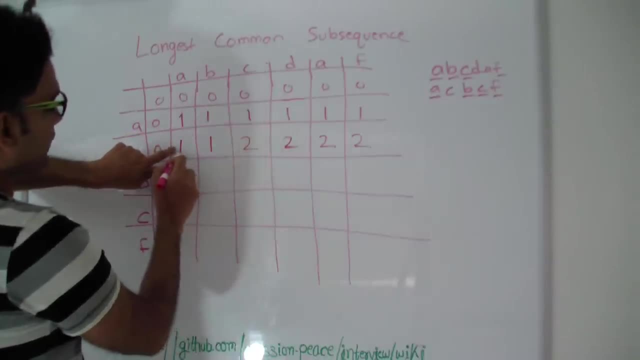 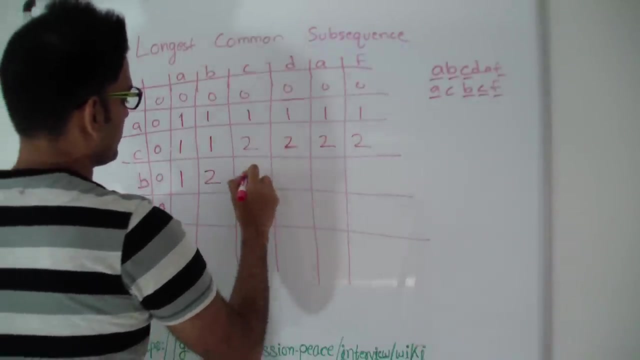 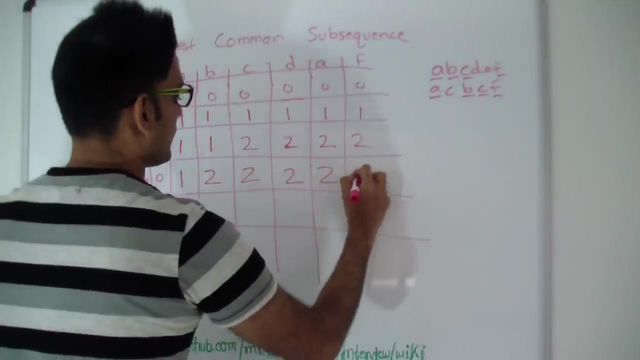 subsequence will be: this guy diagonally cross guy plus 1.. So 2.. Again, b and c are not same, so the length will be max of this two, which is 2.. Here these guys are not same, so max of this two, which is 2.. 2 and 2.. 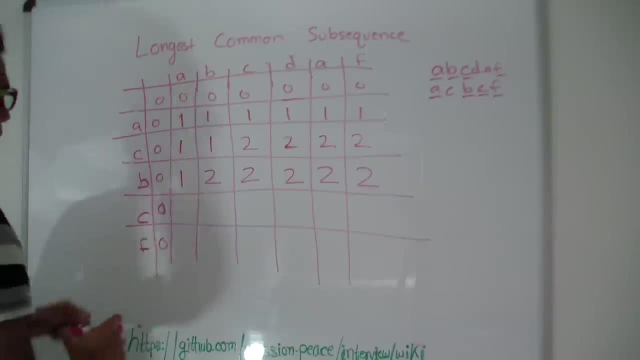 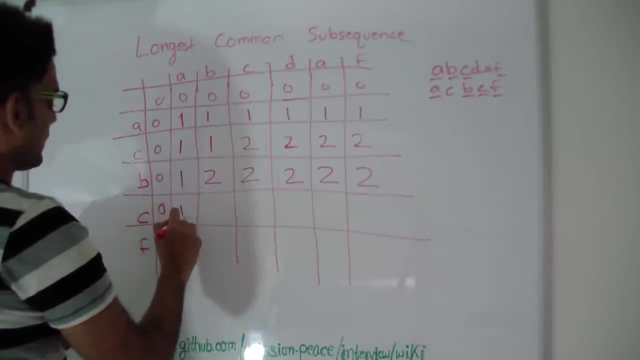 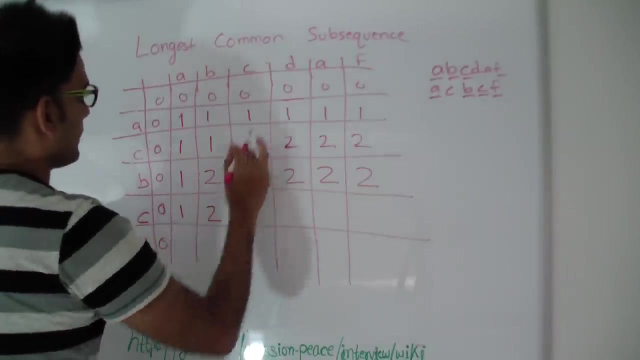 Alright, let's move to the next row. So here we have c and a and they're not same. so the value from the top is 1.. Here c and b are not same, so value from max of this or this is 2.. c and c are. 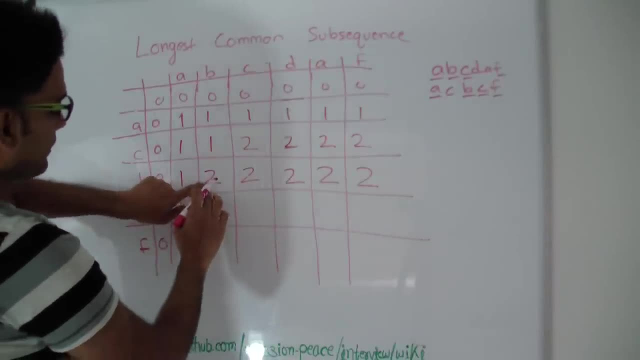 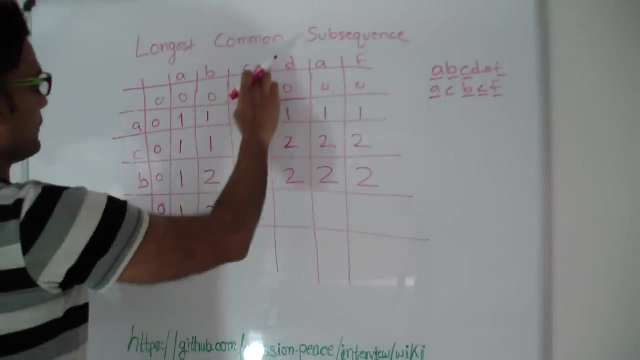 same. so we go diagonally across. so 2 plus 1,3.. Again, when these two guys are same, we are saying is that we already know that these guys will contribute 1 to the longest common subsequence and we'll see the best we can do without. 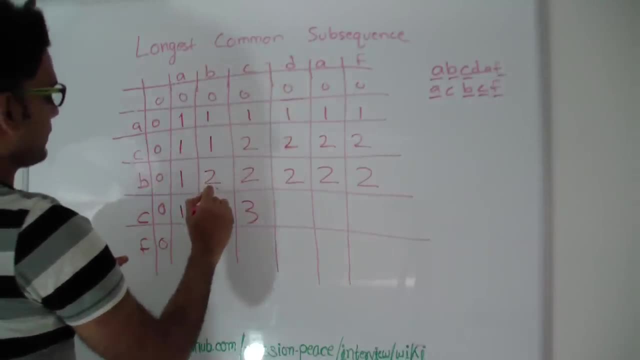 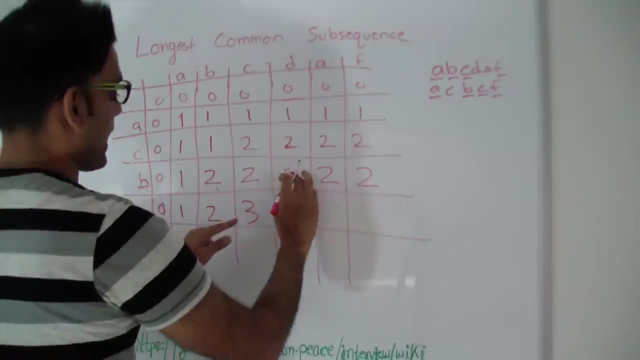 these two guys. So that is ababc, which, well, the number is here 2.. So 2 plus 1,3.. This here is not same, so max of this and this so 3.. They're not same, 3. They're. 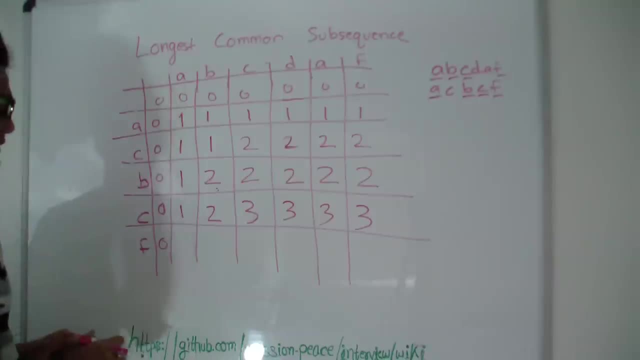 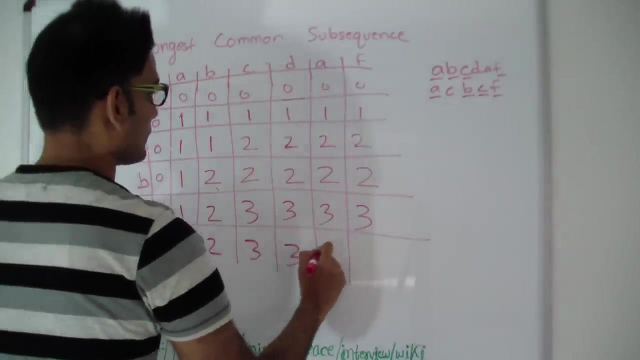 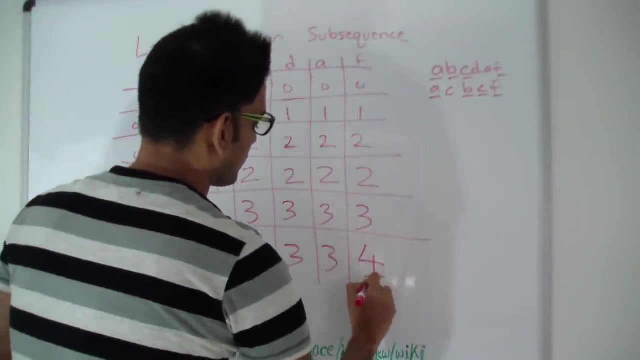 not same, so 3.. Let's finish the fill up the last row, So 1,2,3,3,3.. Since these two guys are same, so the value will be 3 plus 1,4.. So this is the length of our. 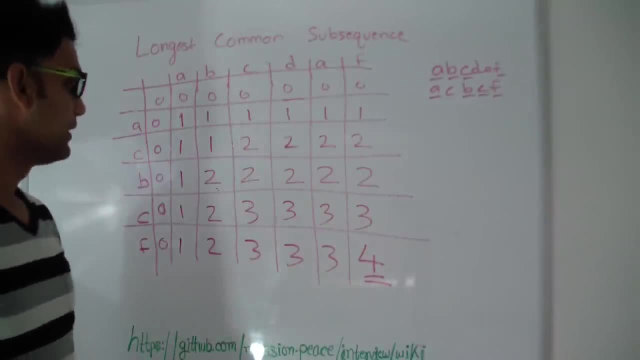 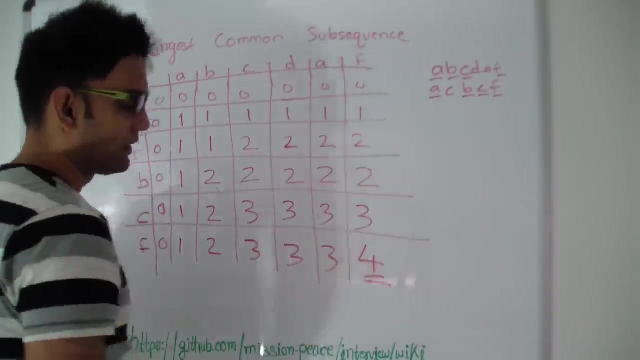 this is the length of the longest common subsequence between them. Now, if you want to find what that actual subsequence is, we'll do this. So we'll start from here and we'll see where this 4 is coming from. So this 4 is not coming from these two guys, So it got to be coming from here. 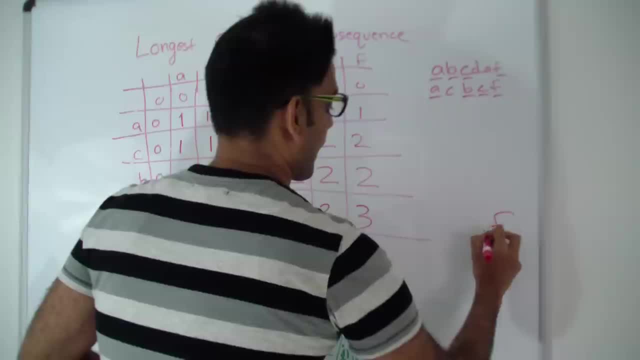 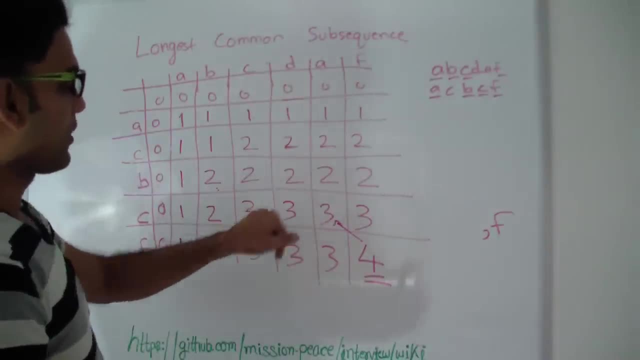 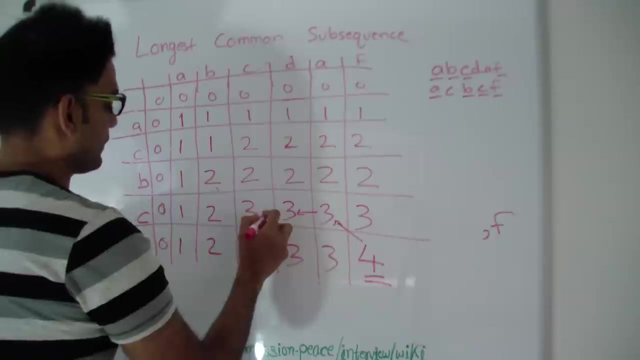 So we know that f is in the answer, So we move here 3.. Where is this 3 coming from? This 3 is coming from here, so we move one step here. Where is this 3 coming from? This 3 is coming from here, so we move one here. 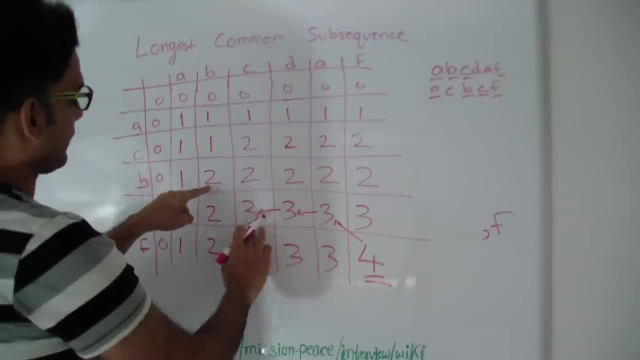 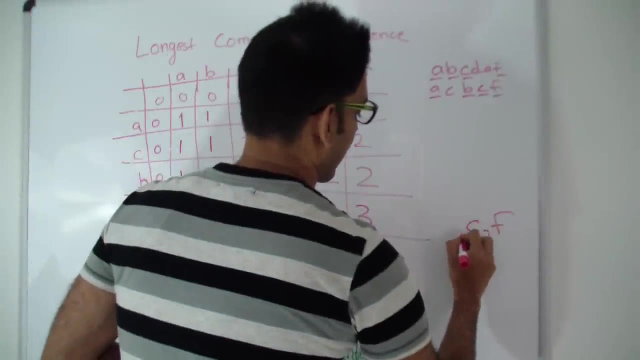 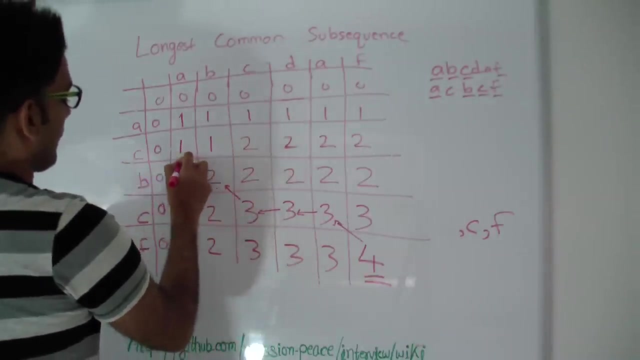 Where is this 3 coming from? This 3 is coming from here, so we move diagonal, and whenever we move diagonal, we include that character c. Where is this 2 coming from? This 2 is coming from here, so we'll include b. And where is this 1 coming from? 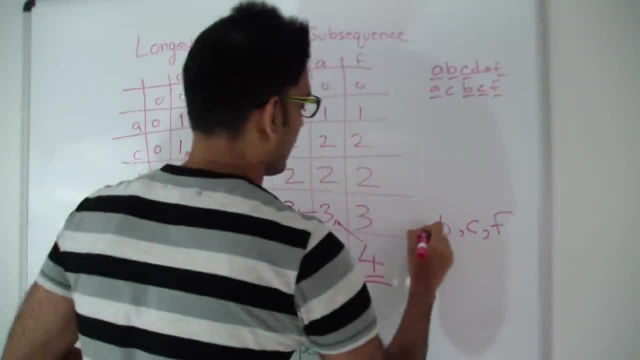 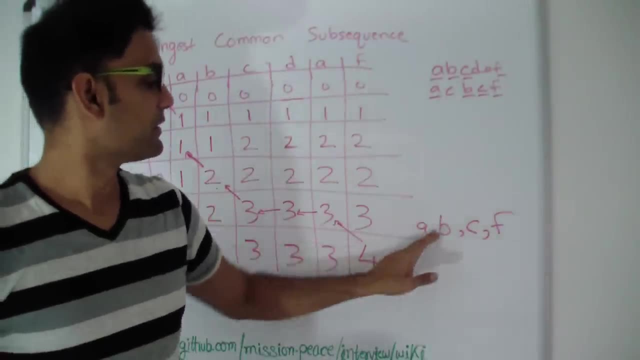 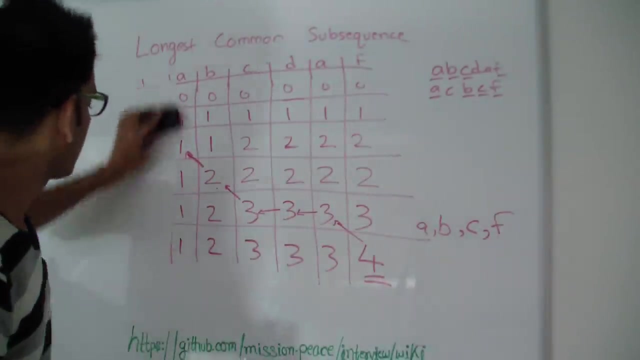 Top. and where is this 1 coming from Here? so we'll include a. Alright. so this is the final result: a, b, c and f is our longest common subsequence and the length is 4.. How would the formula look like? Let me quickly write the formula.